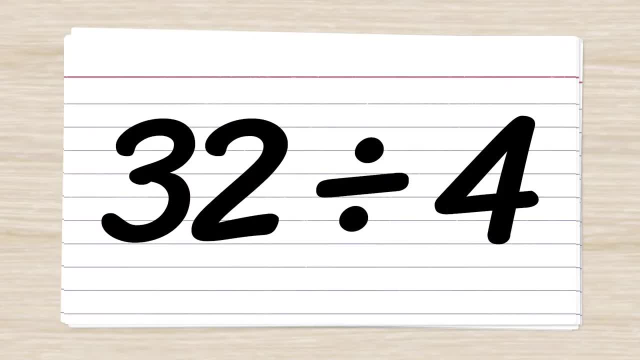 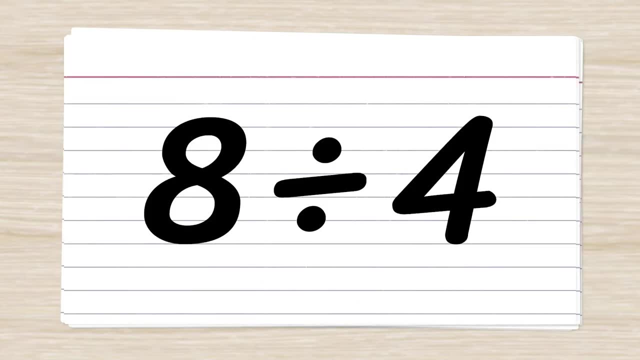 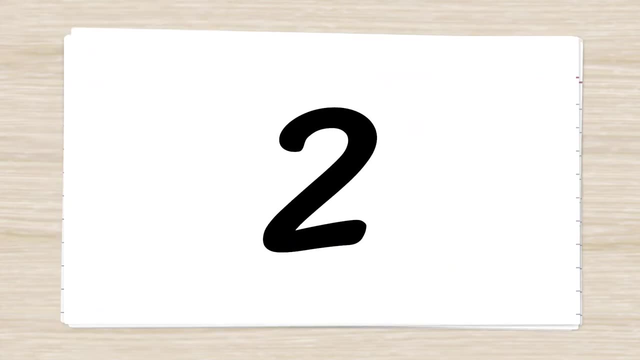 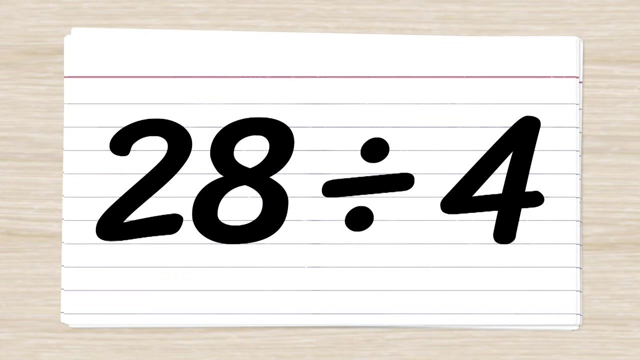 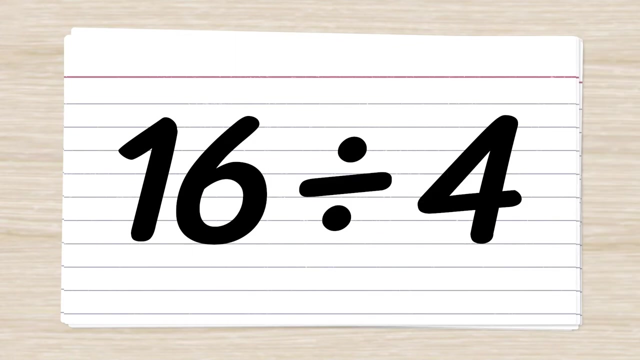 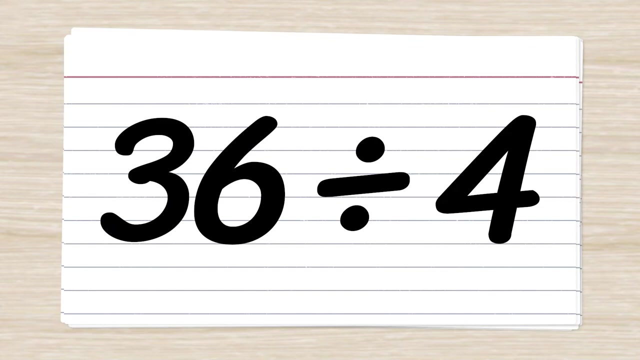 Thirty-two divided by four. Eight. Eight divided by four. Two Forty divided by four. Ten Twenty-four divided by four. Six Twenty-eight divided by four. Ten, Seven, Sixteen divided by four. Four Thirty-six divided by four. Nine Thirty-two divided. 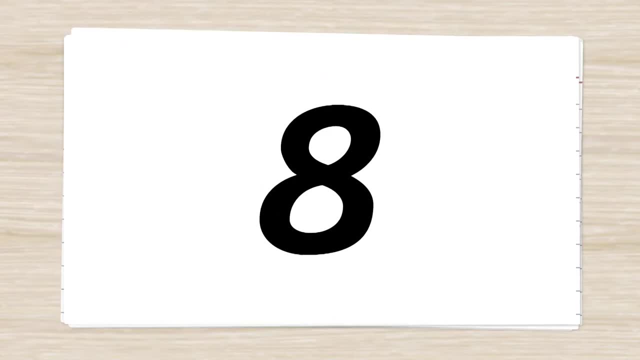 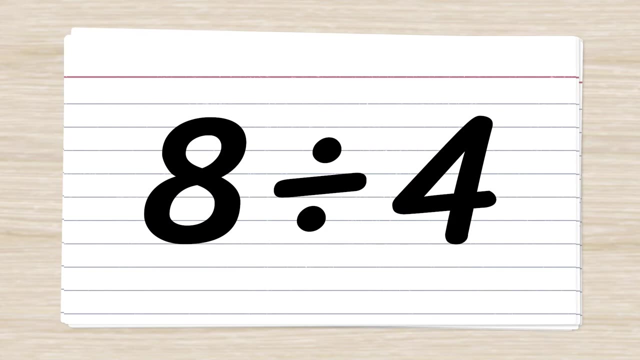 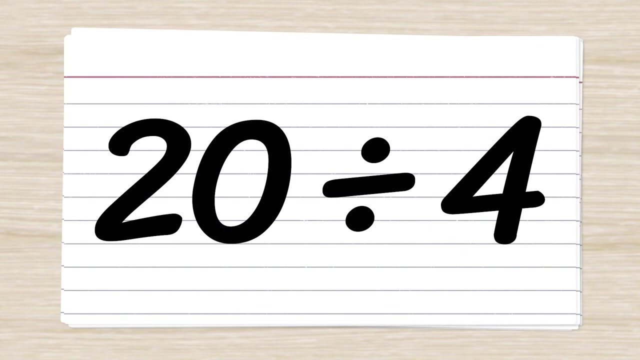 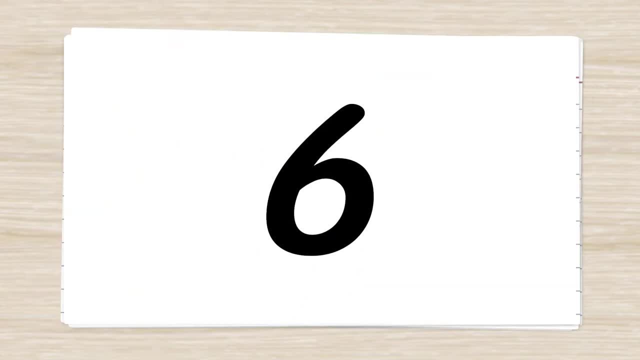 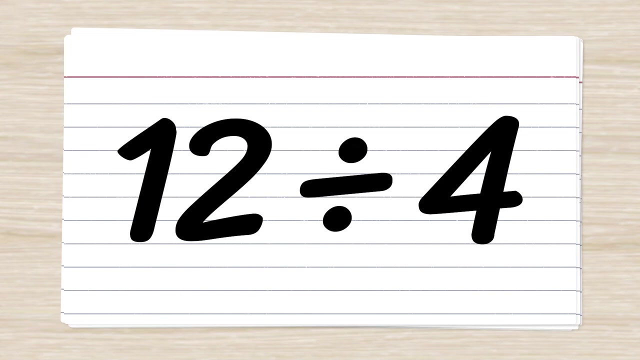 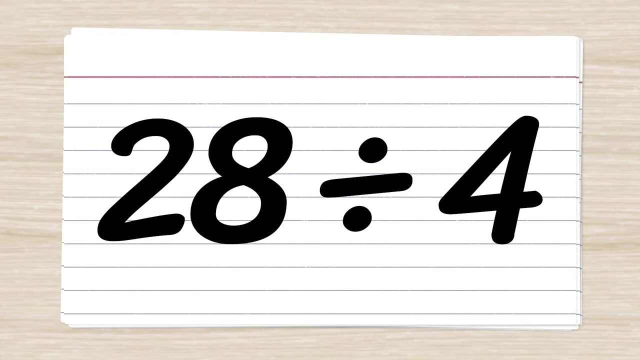 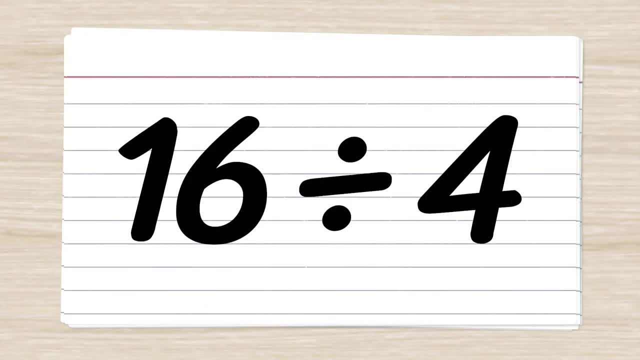 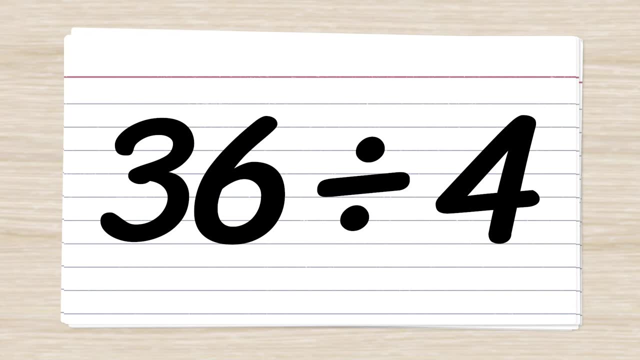 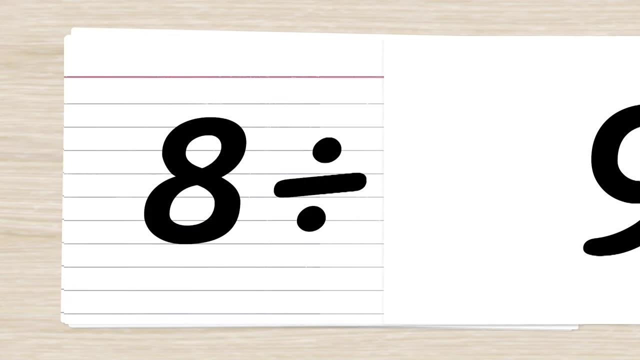 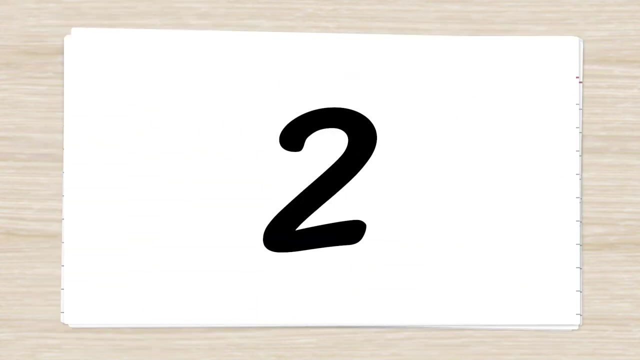 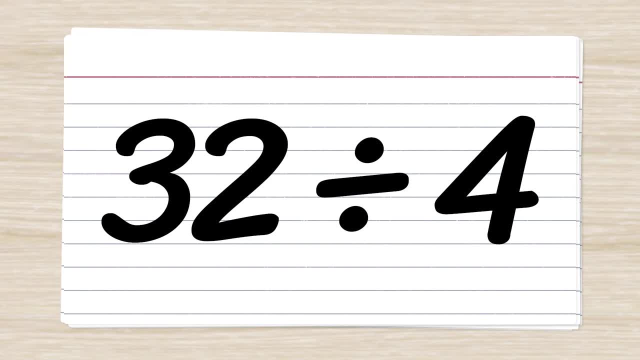 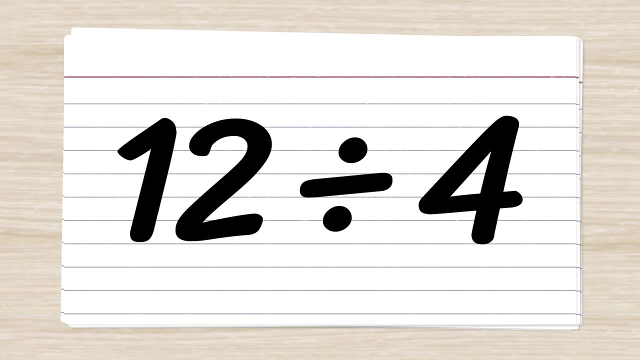 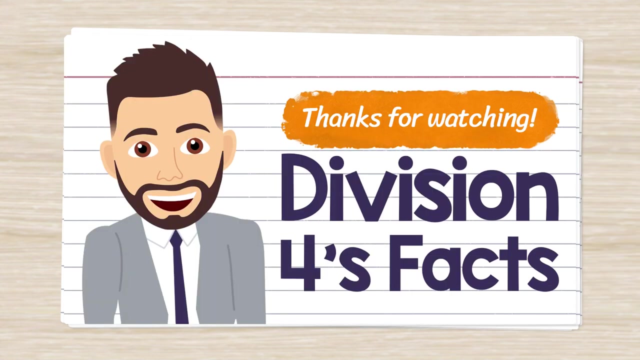